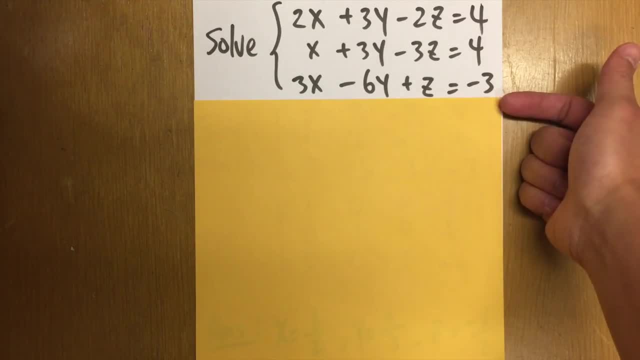 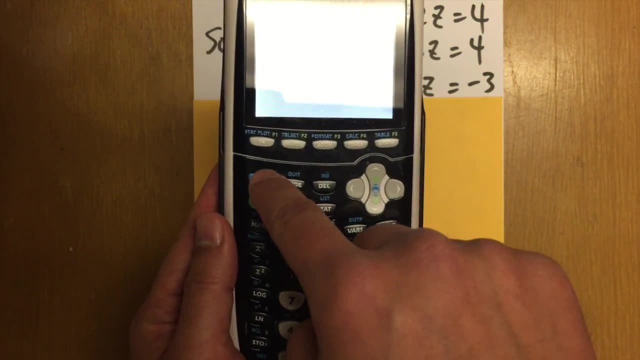 Ding, ding, ding. Hi, We are going to see how to solve this system of equations with the matrix function on TI-84.. First we see that here's the matrix and it's in blue. so we have to hit second and go to matrix. These are the names of the matrices, but then we are going to first go to. 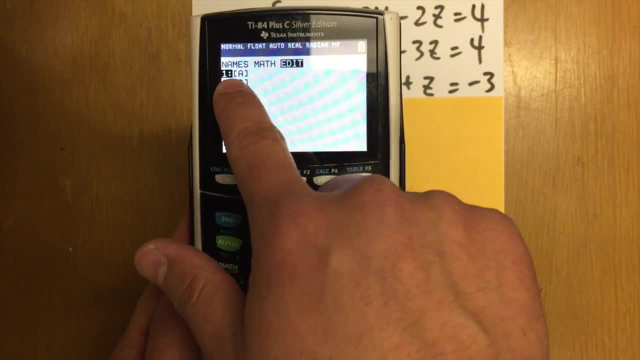 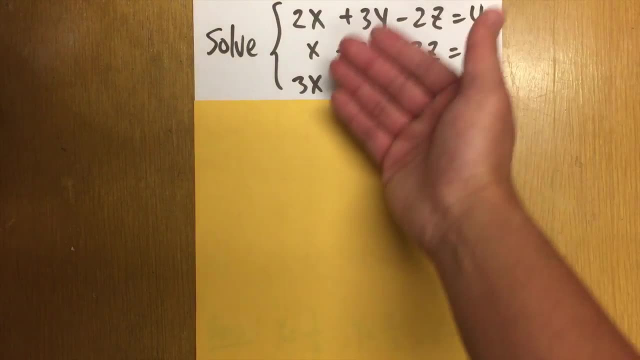 edit first, and then we are going to just say: let's choose the first one so that we can enter our matrix to be matrix A. So let's do that And this is the system of equations that we have. It's a 3x3 system of equations because we have three unknowns and three equations. right. 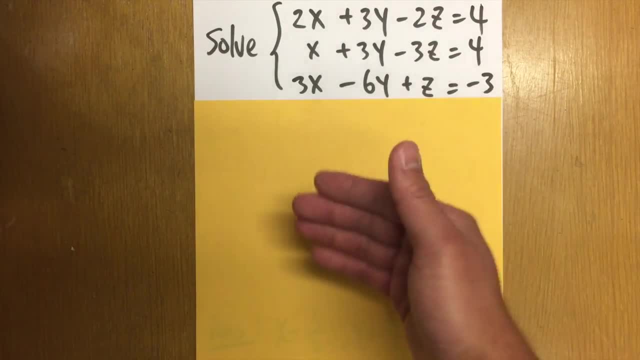 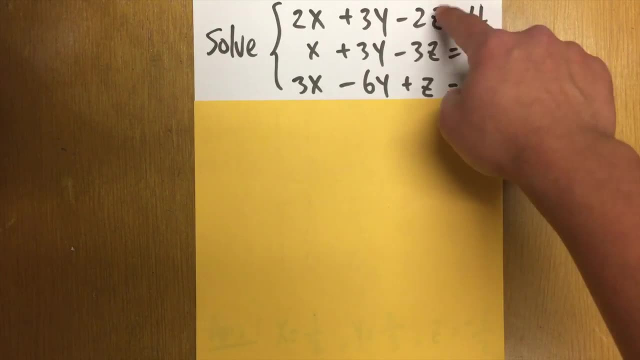 However, when we write this down as a matrix, we will end up with a 3x4 matrix. To do that first, we see that we have to line up with all the x's, all the y's, all the z's, all the equal. 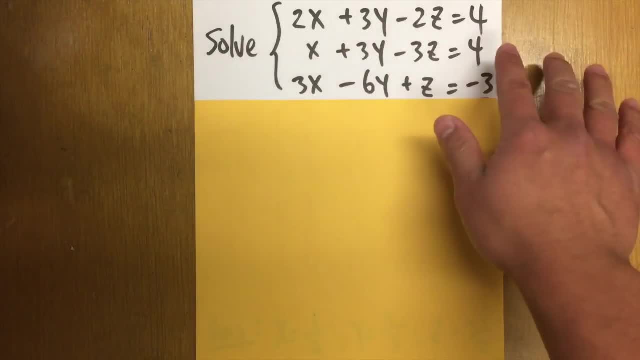 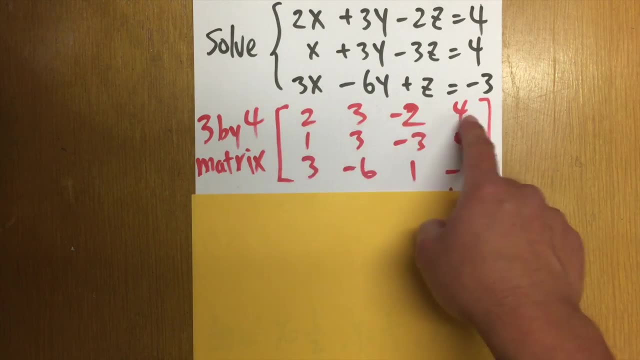 signs and all the numbers, And then we just have to write down the coefficients and we'll end up with this 3x4 matrix. So, for example, the first row, these are just the numbers right here we have the 2, here 3,, negative 2, and 4.. And then for the second row, we will have 1,. 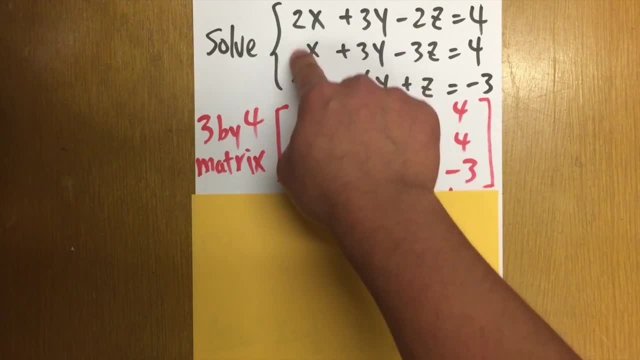 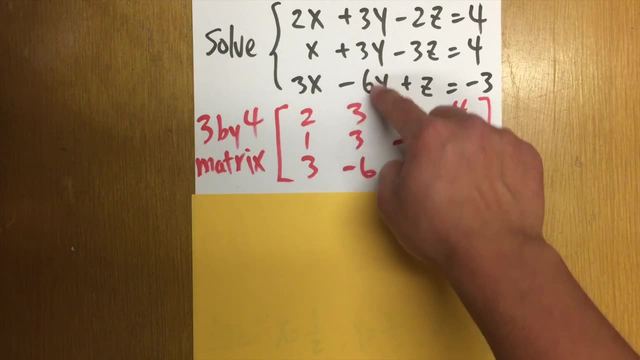 because that's the coefficient in front of the x. right, The number in front of the x is 1.. And then we have 3, negative 3, and 4.. And for the last row we have 3, negative 6,. 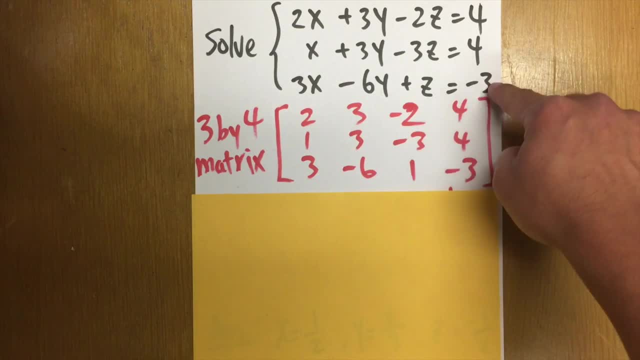 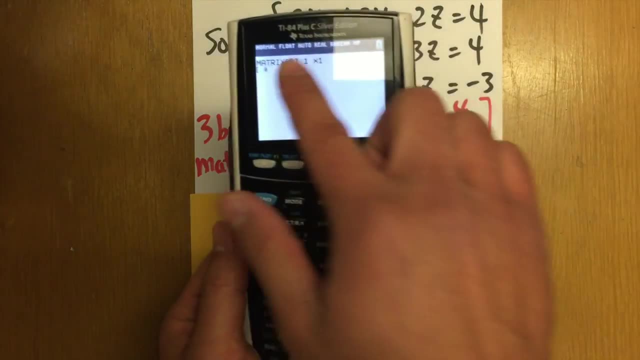 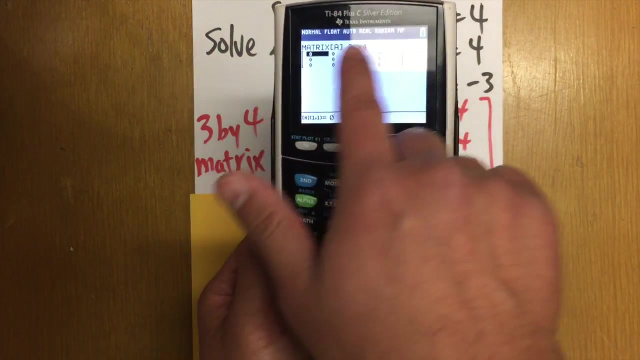 and once again the coefficient of z is 1, and then we have negative 3.. This is a 3x4 matrix, and this is the one that we have to enter onto matrix. First, we are going to make sure we write this down as 3x4. And then we just have to fill in. 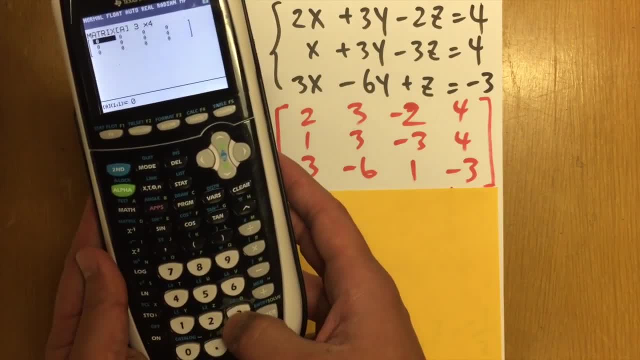 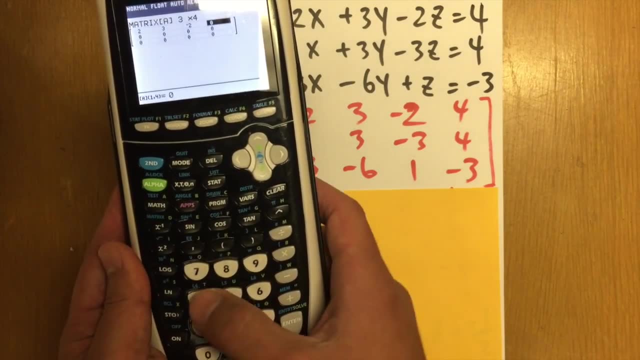 these numbers to be these. So we are just going to do that. So I'm going to put down 2,, 3, and use this for negative, negative 2, and then we have 4.. And then we're just going to continue. 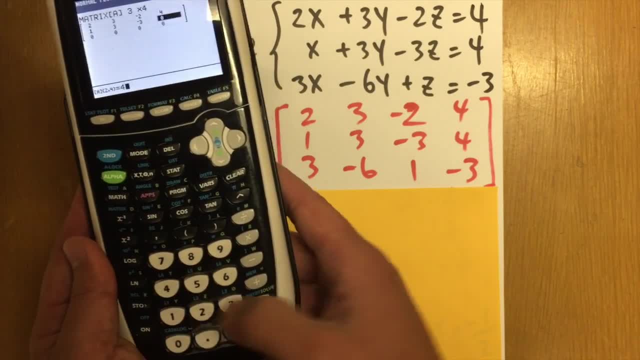 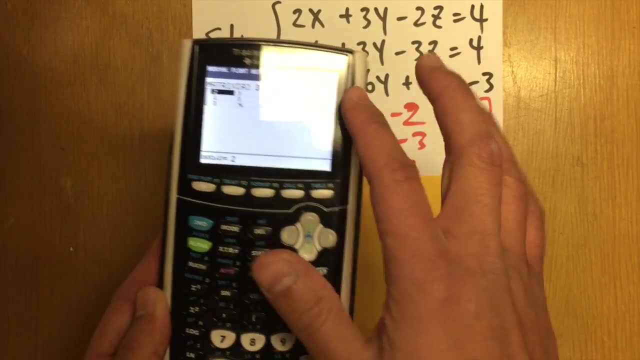 we have the 1,, 3, negative 3, and 4, and then 3, negative 6,, 1, and 3.. Negative: 3,. okay, So, after we fill in the matrix A to be this, this is what we have to do. 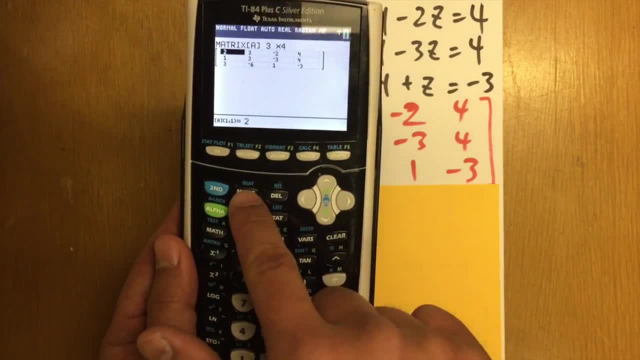 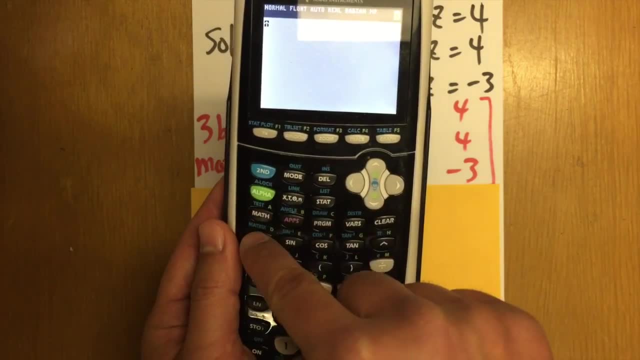 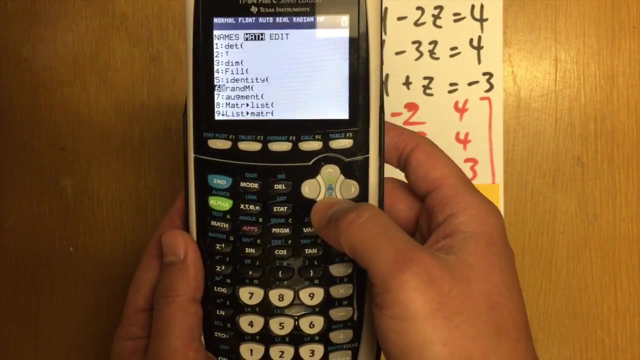 We have to go back home first. Second quit: We have to go back to the home page, all right. And then we are going to go back to the matrix again. Second matrix, But this time we are going to go to math because we are going to do the computations right. We are going to go down to 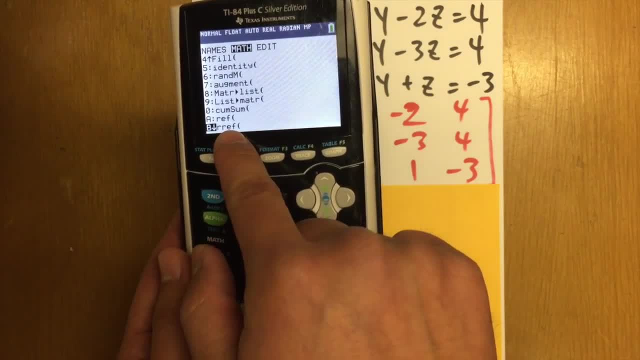 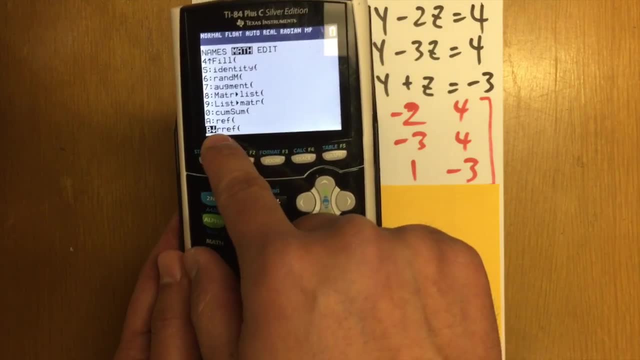 choice B R R E F. This stands for: it will tell you the answer. okay, It will tell you the answer. Don't use R E F. Use R R E F. These two look similar, but then be sure you use choice B R R E F, So select that. 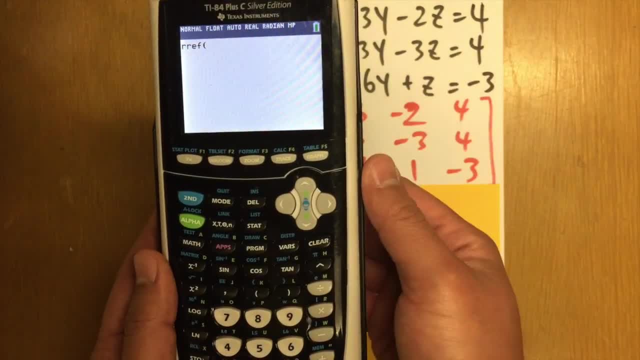 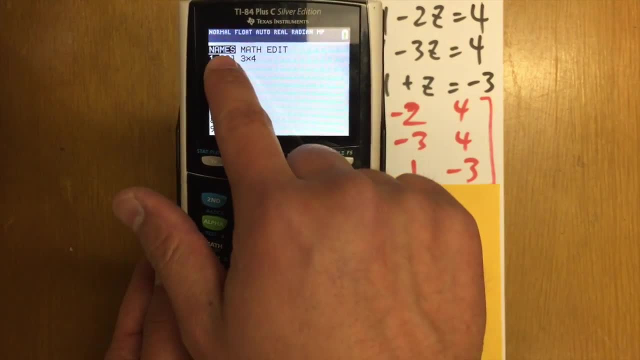 and then we have to enter the matrix that we put in, which is the matrix A, right. So go back to second matrix again, right here. This time we're going to select the first one, which is the matrix A, the 3x4 matrix that we enter the R R E F. So we are going to go back to the matrix again. 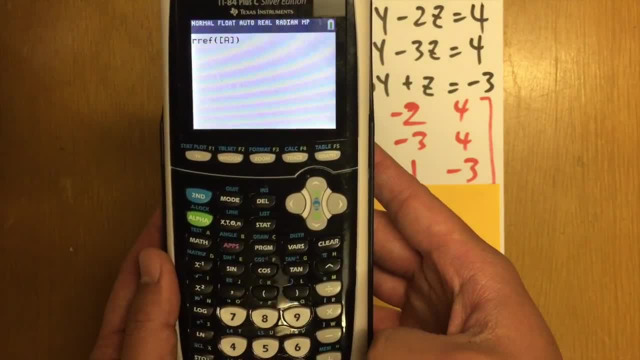 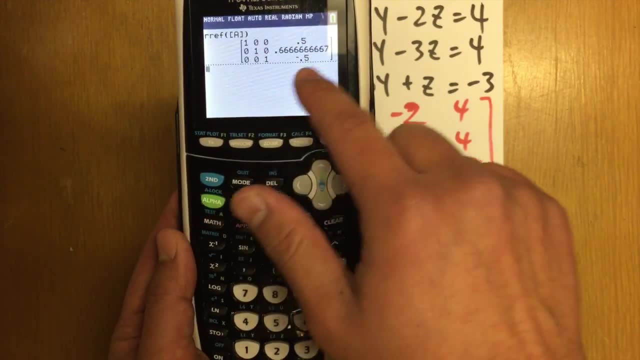 if you did the math earlier, and then we are going to close the parenthesis and we are just going to hit enter once again, like this: As you can see, this is in the R R E F form: 1,, 1, 1 on the. 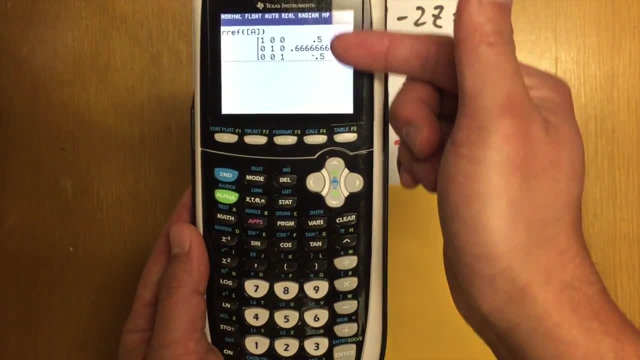 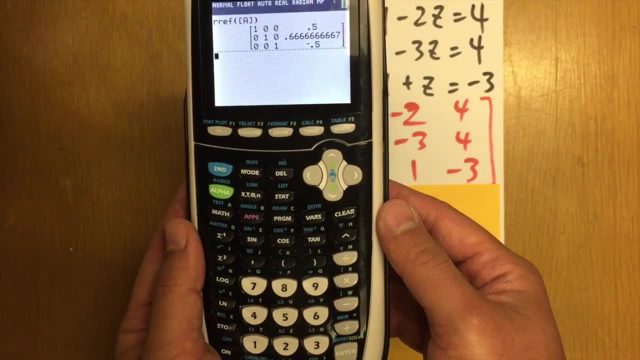 diagonals, and then you have all the zeroes right here and these are the answers. But then these are the decimal numbers, right? That's not so good. This is how we can do. We are going to go to math and then just select the first one. 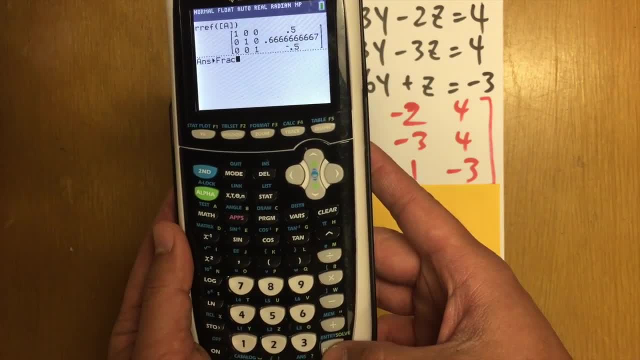 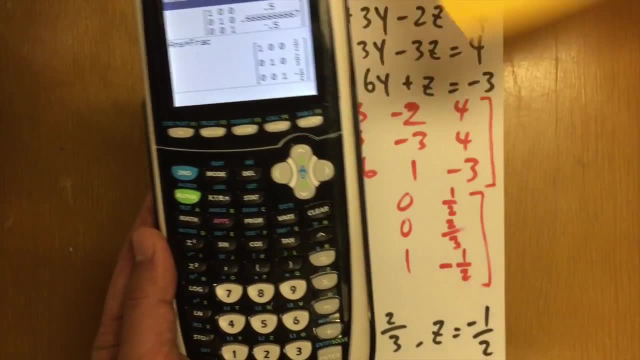 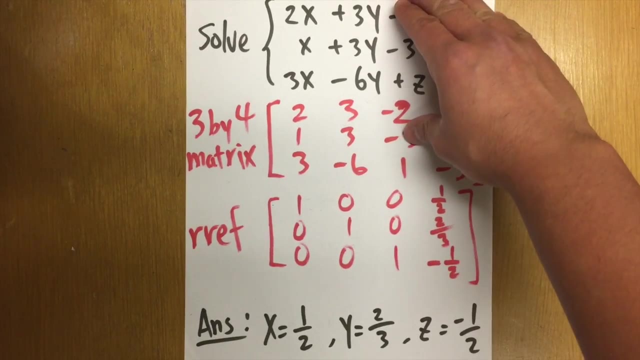 so we can change the decimals to fractions. Let me show you. You see, this is the RREF with fractions, and this is pretty much what we have right here. So RREF just means that we are going to have the matrix, where the diagonals are. 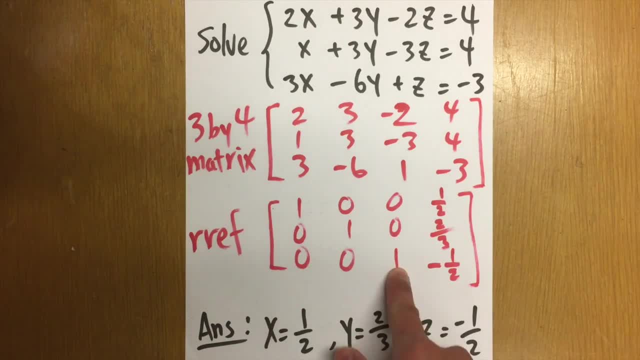 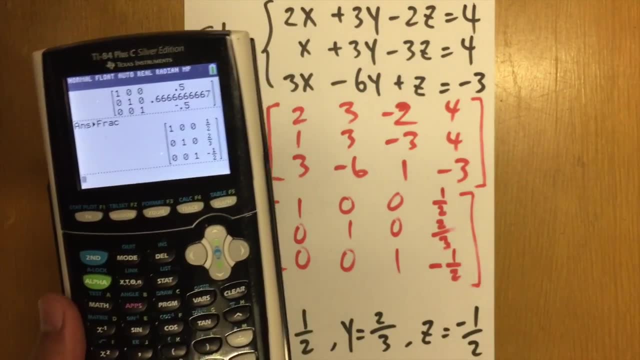 1, and this is the good situation. We have all this 1 right here, and then we have 1 half, 2 thirds and negative 1 half right, And this is how we are going to read the answer. This is the x column. We have 1x, no y, no z, and this right here. 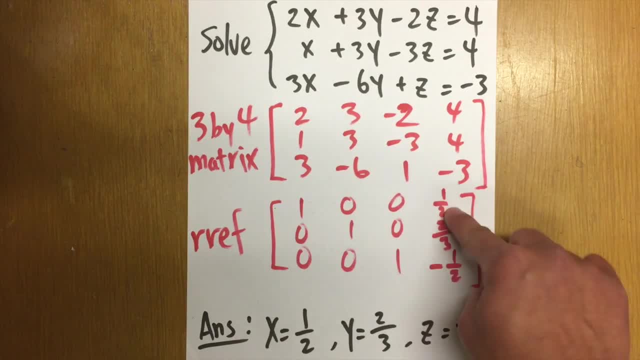 is 1 half. That means 1x is equal to 1 half, so x is equal to 1 half. Likewise, this right here is the y column, so that means we have 0x, 1y, 0z and this is: